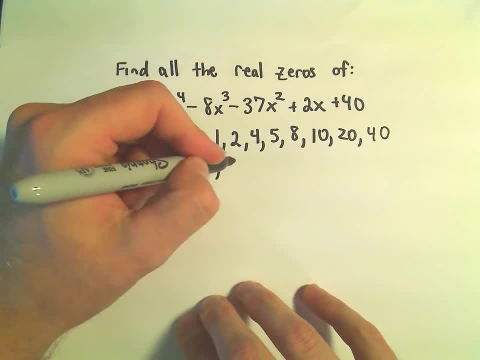 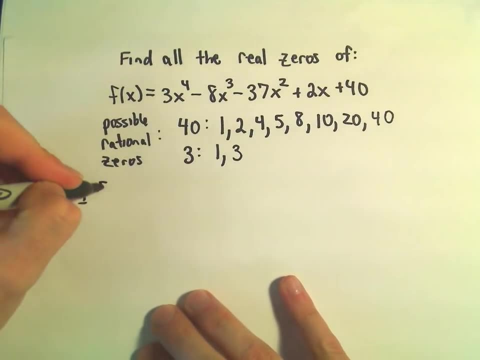 Then we look at factors of the leading coefficient, which is 3. So the factors there would just be 1 and 3. And then it says all the possible rational zeros. We get positive and negative, all the numbers that I'm about to write. 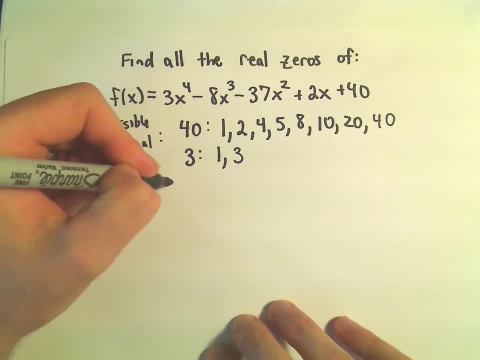 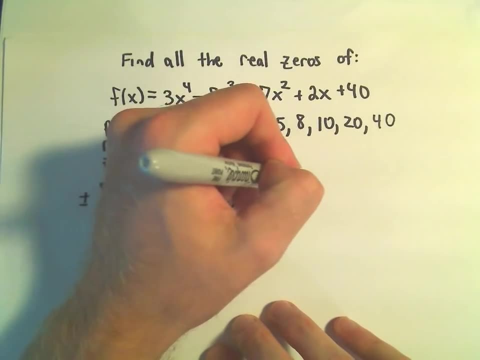 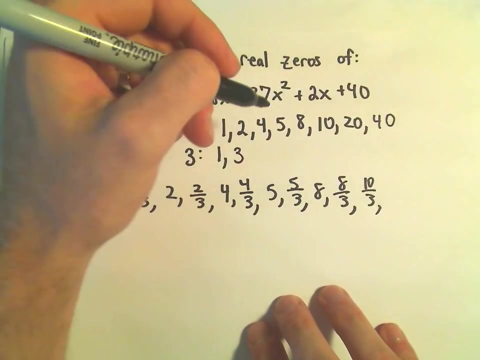 So 1 over 1, 1 over 3,, 2 over 1, 2 thirds. We could have 4 and 4 thirds. We could have 5, 5 thirds. We could use 8 or 8 thirds, 10, 10 thirds- Let's see 20, 20 over 3.. 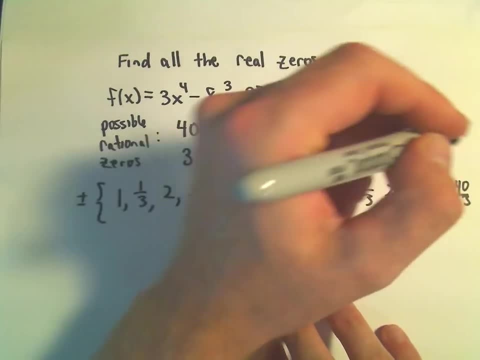 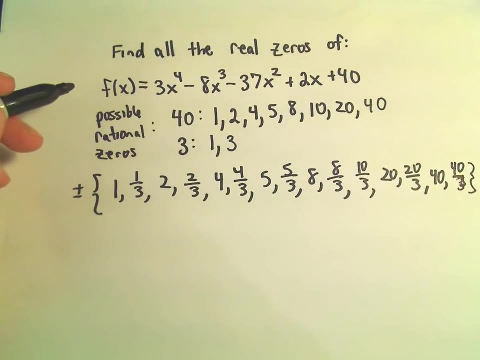 We could have 4. 40 or 40 thirds- Any of those numbers could be possible- rational zeros. So what I'm going to do now is use the remainder theorem because, again, if we plug one of these numbers in and get 0 out, that means it's a factor. 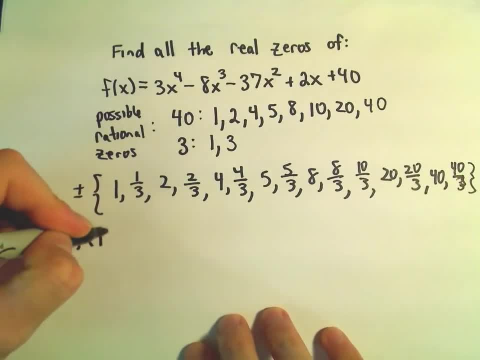 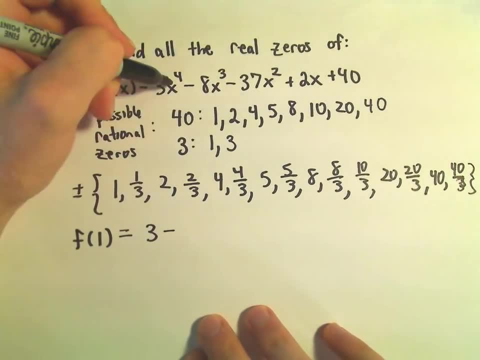 So I'm just going to start off with the easiest one and I'm going to plug 1 in. So if we plug 1 in, we'll get 3.. You know, if you plug 1 in anywhere for the x, we'll just get 1.. 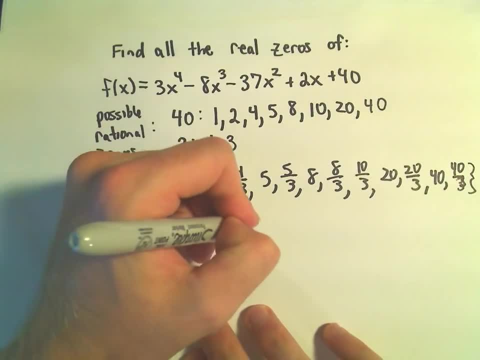 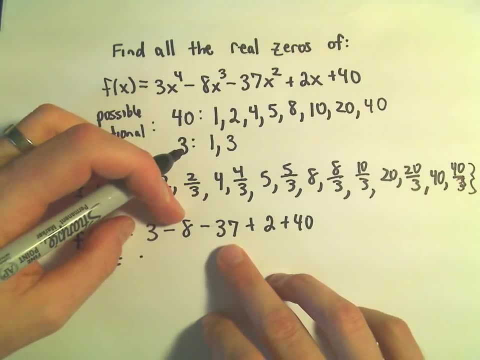 So we'll have 3 minus 8.. Minus 37 plus 2 plus 40.. Well, 3 minus 8 is negative 5.. Negative 5 minus 37 would be negative 42.. Positive 2 and positive 40 would be positive 42.. 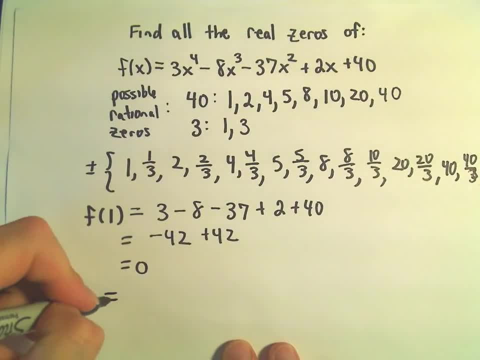 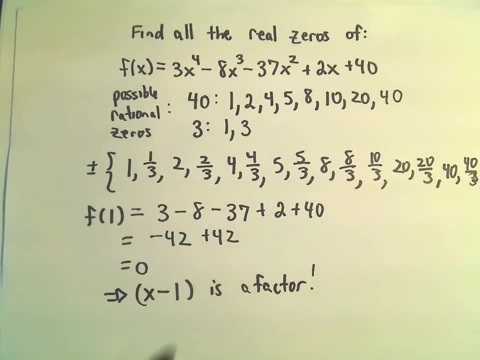 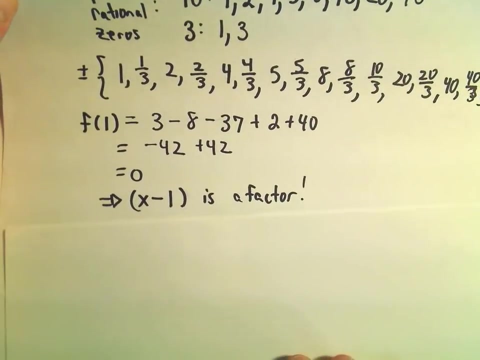 So, hey, we get 0 out. So again, this tells us that x minus 1 is a factor, And I'm going to factor my polynomial now using long division Or not long division. We could do long division. Let's use synthetic division. I think that's a bit easier. 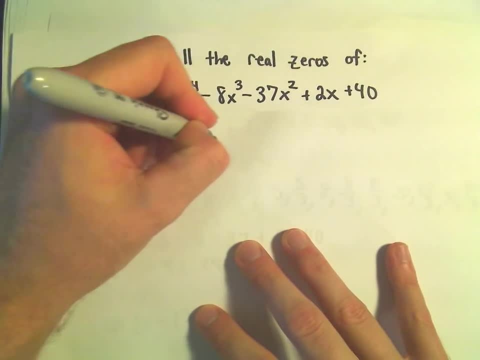 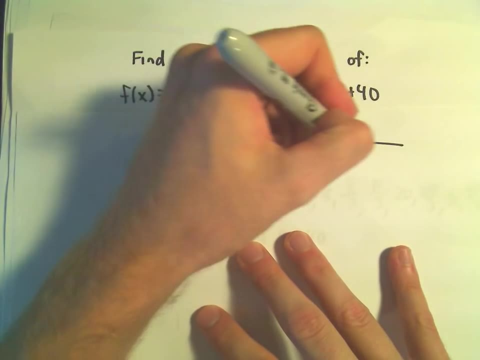 So again, synthetic division. we just write down the coefficients, So we've got a positive 3, a negative 8, a negative 37, a positive 2, and a positive 40. We said 1, x minus 1 is a factor. 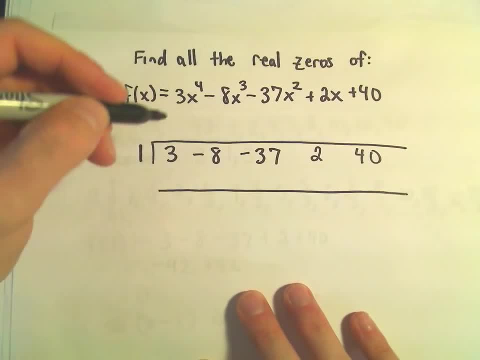 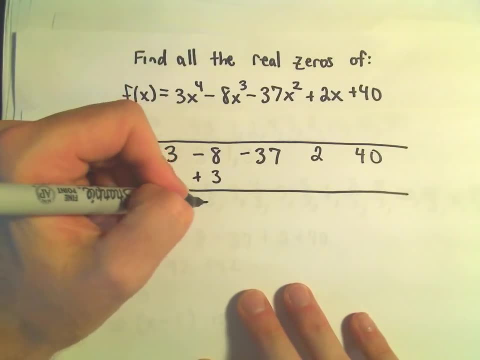 So we just put a positive 1 outside Again, that was our 0. And then we just drop down the first number. So 1 times 3 is 3. And then we just add, So we'll get negative 5.. 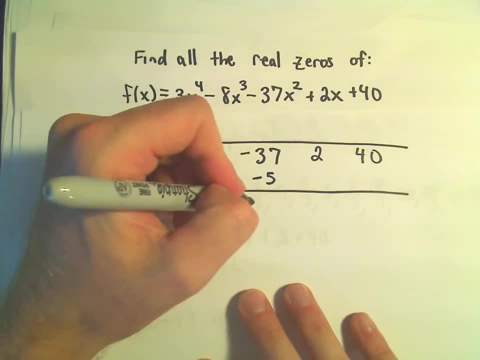 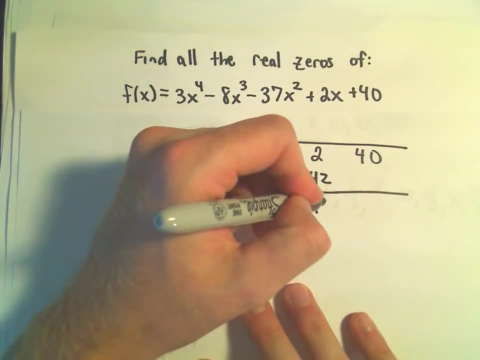 Then we multiply, So negative 37 and negative 5 is negative 42. Again, we just drop that one over. If we add, we'll get negative 40.. 1 times negative 40 is negative 40. We get 0 as our remainder. 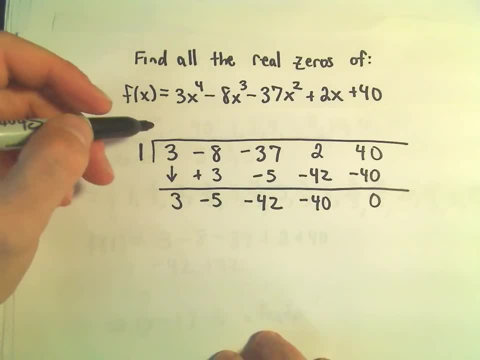 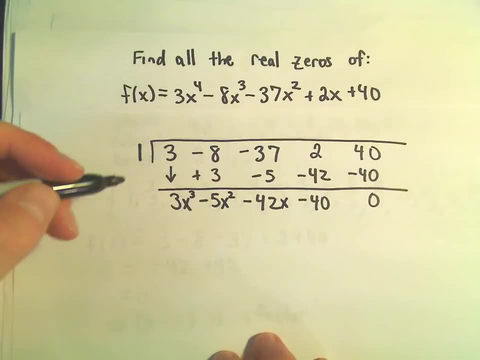 Which, again, we should be getting if 1 is in fact a 0.. We started with something x to the 4th, So this will be 3x cubed. This will be our x squared, Our x term and our constant. 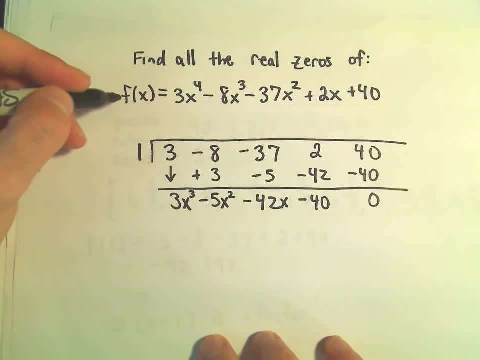 So it says our original polynomial f of x, 3x to the 4th minus 8x, cubed minus 37x, squared plus 2x plus 40. It says we can really write our original polynomial as x minus 1.. 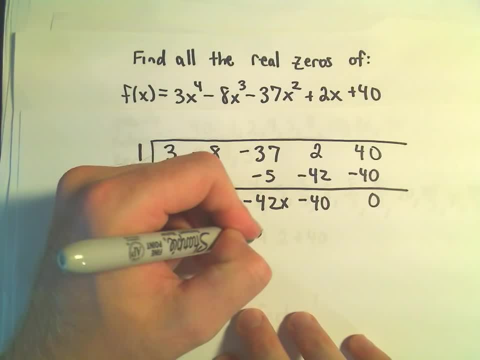 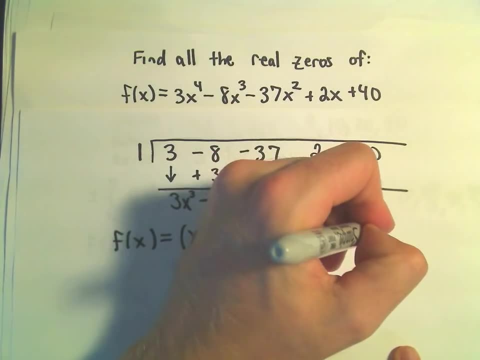 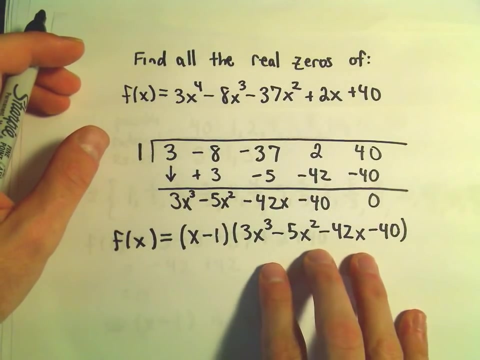 That was our 0. So we knew that was a factor Times: 3x cubed minus 5x squared minus 42x minus 40.. So now what I'm going to do is I'm going to try to break down this factor, this 3x cubed factor, minus 5x squared minus 42x minus 40.. 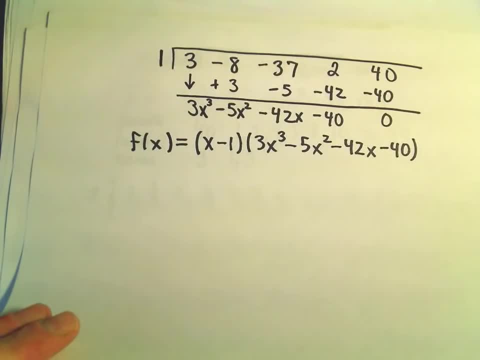 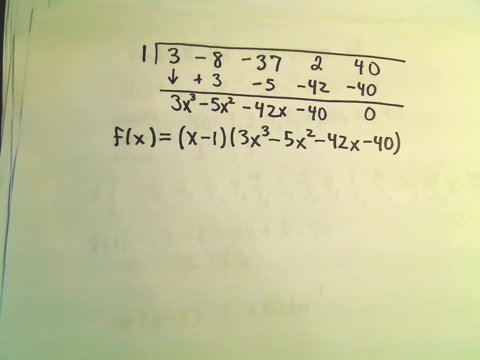 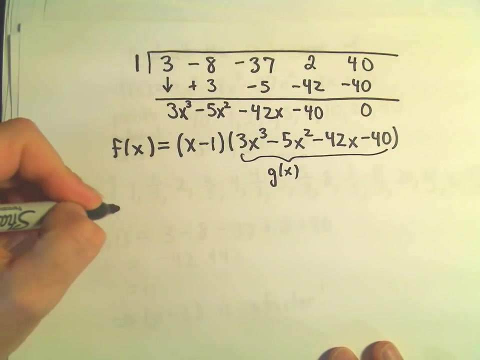 I'm going to try to break that one down a little bit more. So, again, we've got all these sort of possible rational zeros, So what we need to do is just simply find another one that's going to work. So maybe we'll call this function g of x, just because it's something a little different. 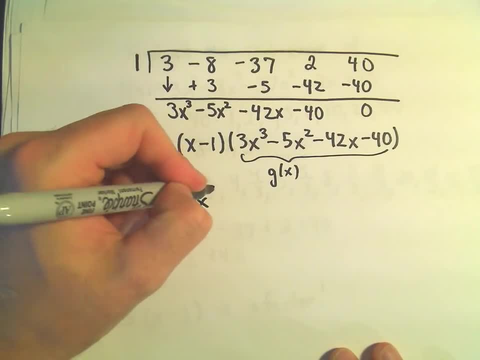 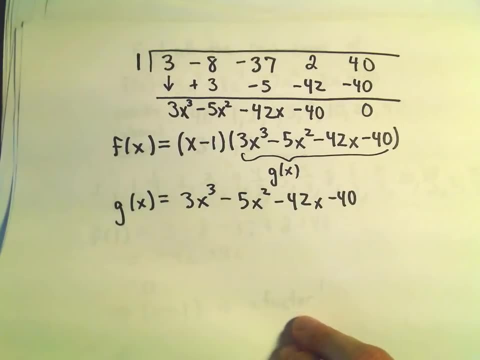 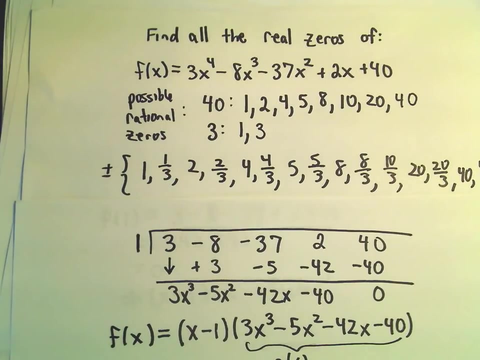 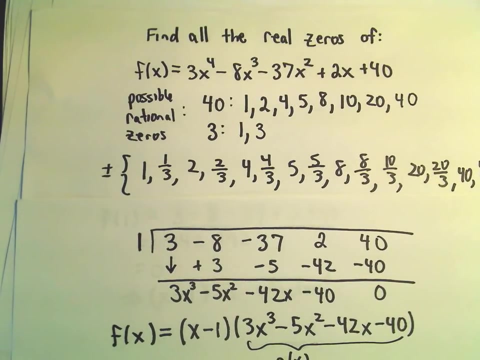 So g is 3x cubed minus 5x squared, minus 42x minus 40.. So again we've got a bunch of different candidates here, We've got all these numbers that we were just sort of testing out here, And what I'm going to do is, again I'm just going to kind of trial and error. 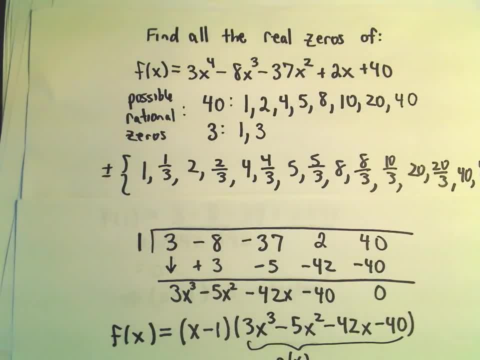 you know, maybe plug in a couple different numbers Again. which one should you use? You know, that's where it gets a little tricky. We could use negative 1, but I think if we use negative 1, I don't think that's going to work at all. 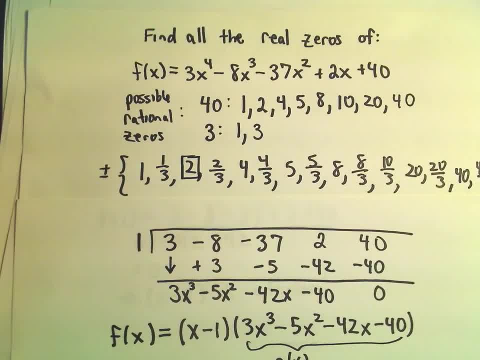 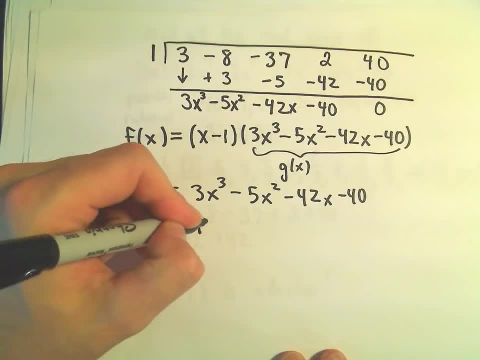 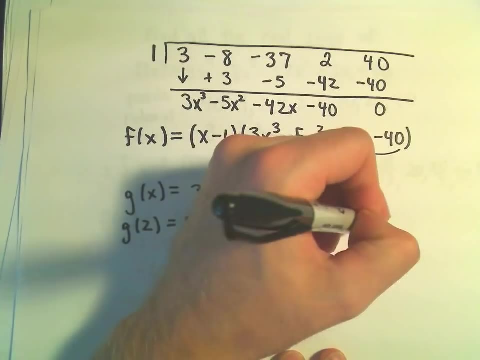 I'm going to jump over to me to use the next easiest number that I think, which will either be positive 2 or negative 2.. So let's see, If we plug 2 in we would get 3x2 cubed minus 5x2 squared, minus 42x2 minus 40.. 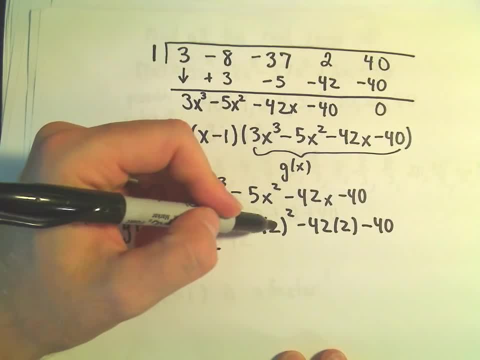 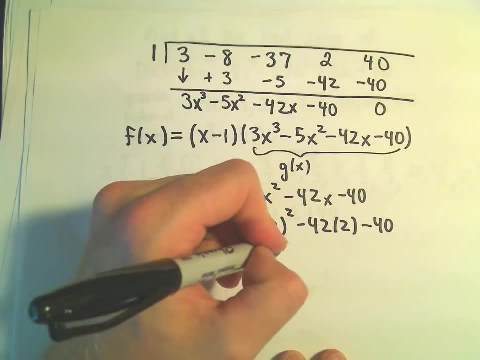 So 2 cubed is 8 times 3 is 24.. 2 squared is 4 times negative. 5 will give us negative 20.. Negative 42 and 2 will be negative 84 minus 40. Well, there's definitely lots of negative numbers out there. 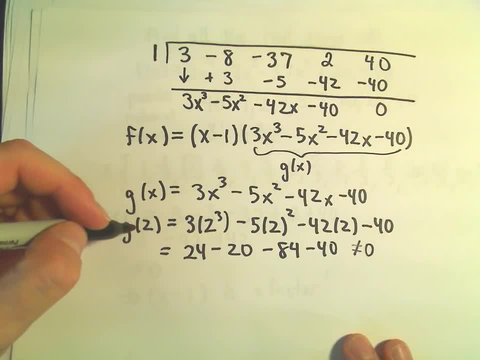 That's not going to equal 0. So that means x minus 2, that's not our factor. Maybe we can check negative 2.. So if I plug negative 2 in we'll get 3 times negative 2 cubed. 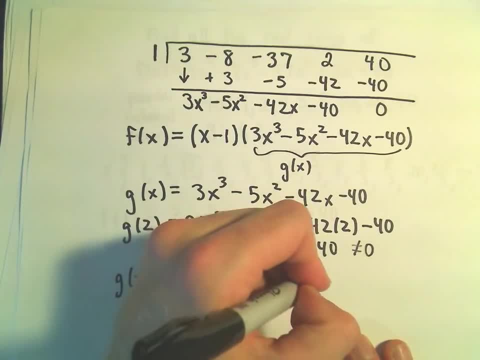 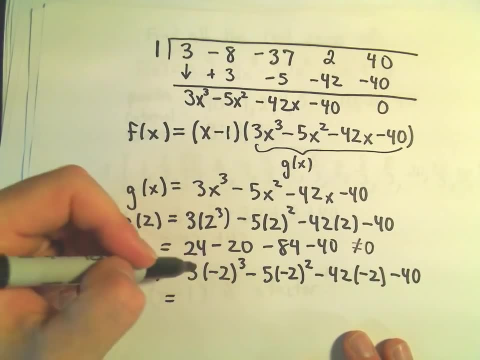 Minus 5 times negative. 2 squared minus 42 times negative. 2 minus 40.. Negative 2 cubed is negative 8 times 3 would be negative 24.. Negative 2 squared is 4 times negative. 5 would be negative 20.. 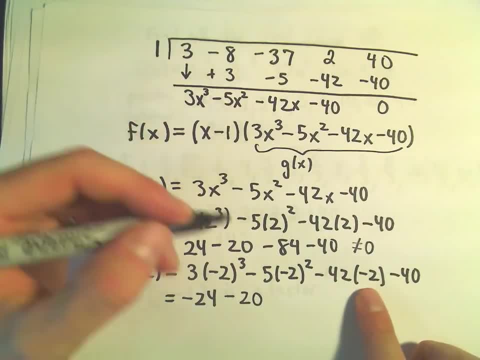 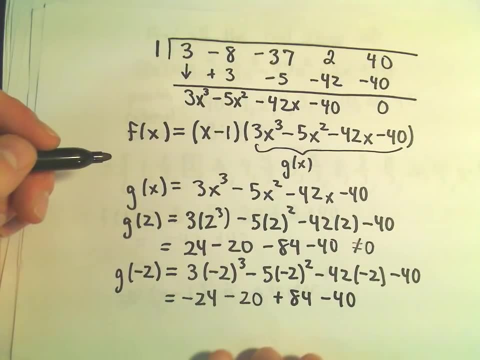 Let's see Negative 42 and negative 2 will be positive 84. And then we've got our minus 40 left over. Hey, I think this one's going to work. Say, if we get negative 24 minus 20, that's negative 44.. 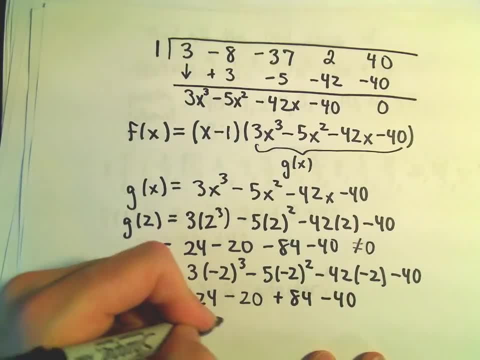 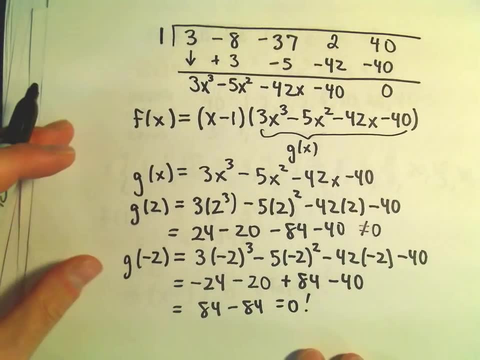 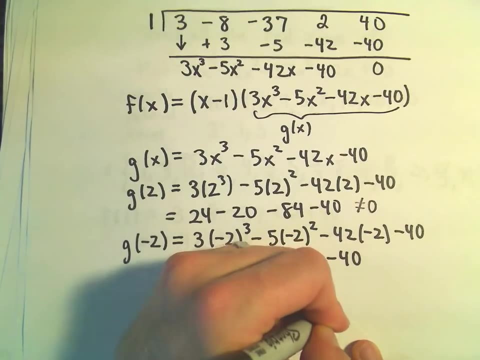 Minus another 40 will be negative 84. So we have 84 minus 84. That gives us 0. That means negative 2 is a 0. And that tells us that x plus 2 is a factor. Okay, great. 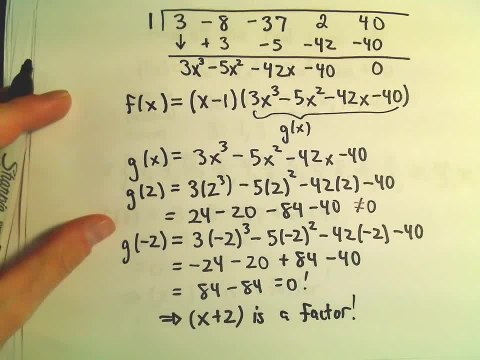 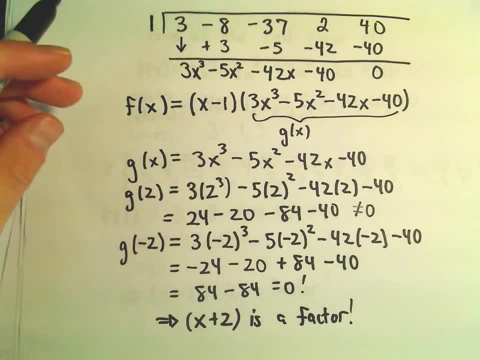 So we know the quantity x plus 2 is a factor. So what I'm going to do now is I'm going to do an aesthetic division on my factor g of x to sort of help us break it down a little bit further. Okay, so I'm going to take the coefficients. 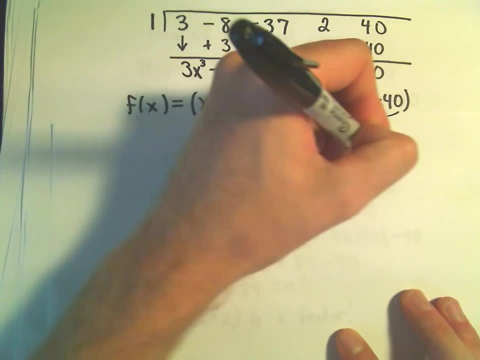 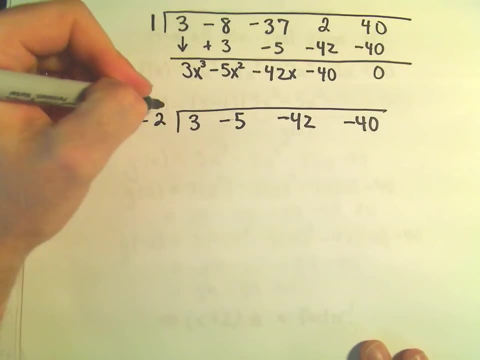 We've got 3, negative 5, negative 42, and negative 40. Again, our 0 was negative 2, so that's what goes on the outside. Let's be careful with our arithmetic. So we just drop down the 3.. 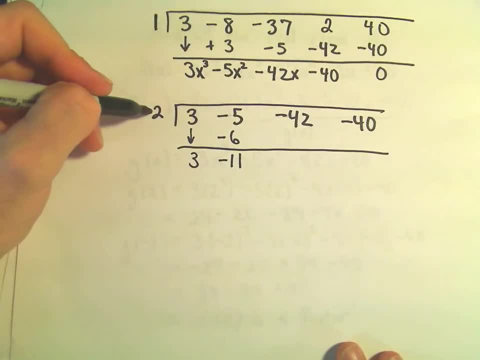 Negative 2 and 3 is negative 6. If we add, we get negative 11.. Negative 2 and negative 11 is positive 22.. Again, if we add, we get what is that? negative 20.. And negative 2 times negative 20 is positive 40.. 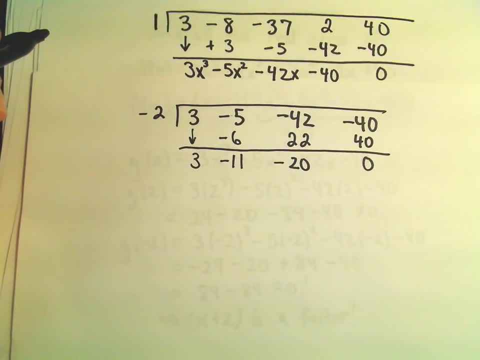 If we add, we get our remainder of 0, just like we should get. So again. we started with something x cubed. This will be our x squared term, This will be our x term and our constant. So what it says is: we're trying to factor f of x again, remember? 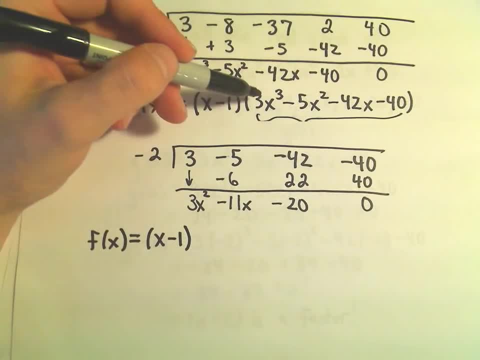 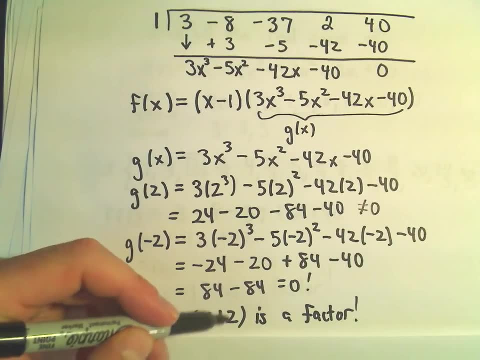 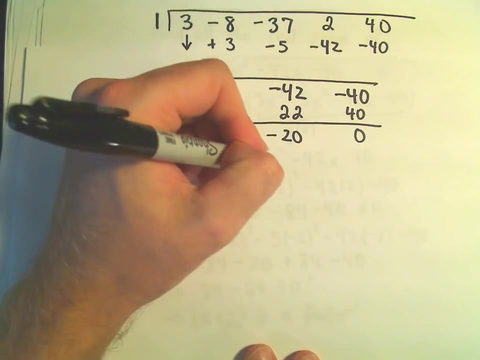 So f of x was x minus 1.. Times this polynomial g of x. But again we said a factor of g of x was going to be x plus 2.. So I'm going to drop in my x plus 2.. And then what would be left over would be our 3x squared minus 11x minus 20.. 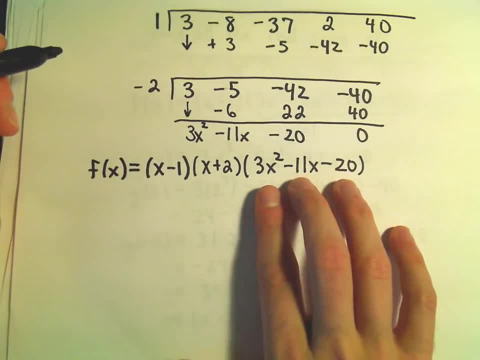 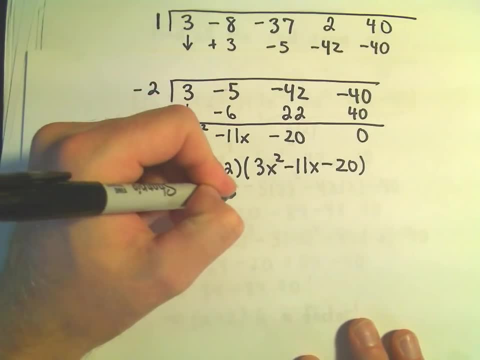 Okay, so we could do two things. Again, we're trying to find zeros. To find the zeros of this quadratic factor, we could always just use the quadratic formula- I'm going to see if I can't play with numbers here- and get it to factor. 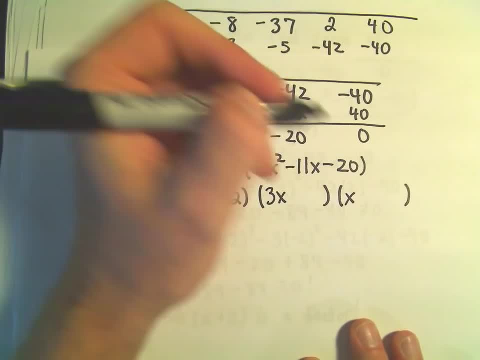 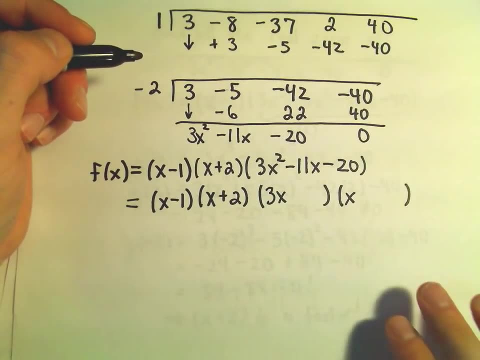 So to get my 3x squared I'm going to need basically a 3x and an x. if I use whole numbers, Let's see What would be some good numbers that might work here. Let's see What if we use 4 here and 5 there. 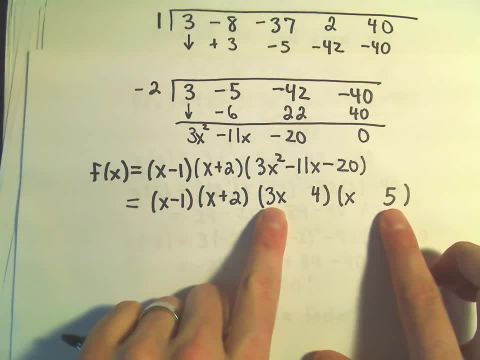 Because that will give me 15 when I multiply. I think we can stick a negative there and a positive there. So let's check. We would get 3x squared minus 15x, plus 4x, which would be negative 11x. 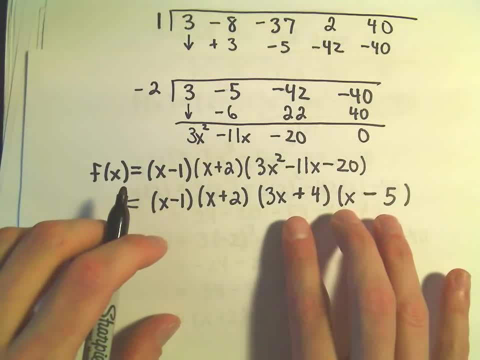 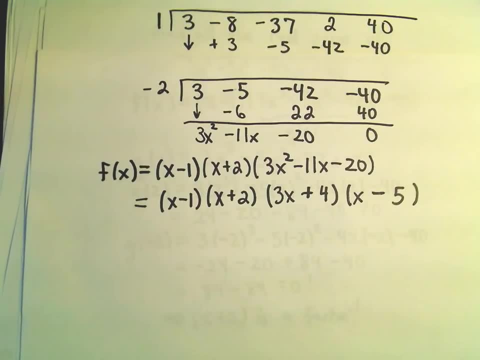 And then we would get our negative 20.. So it looks like to me this: 3x plus 4 times x minus 5 is a correct factorization of our quadratic factor. And, hallelujah, we have now got it factored. 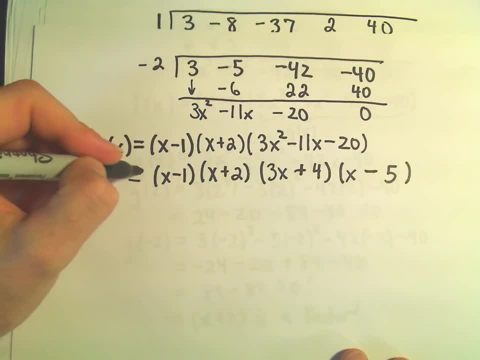 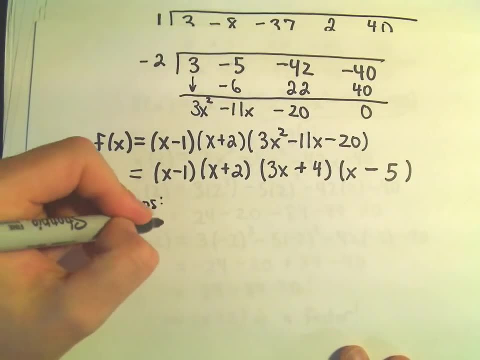 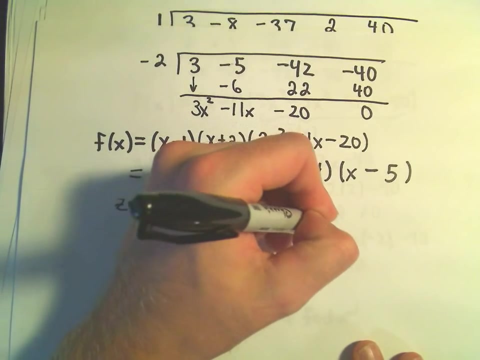 So if we want to find the zeros, if we want to find the zeros again, we just set this whole polynomial equal to zero. So x minus 1 times x plus 2 times 3x plus 4 times x minus 5 equals zero. 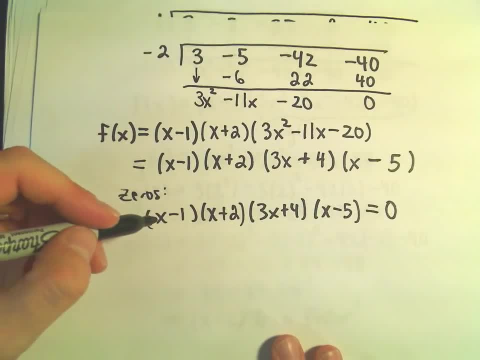 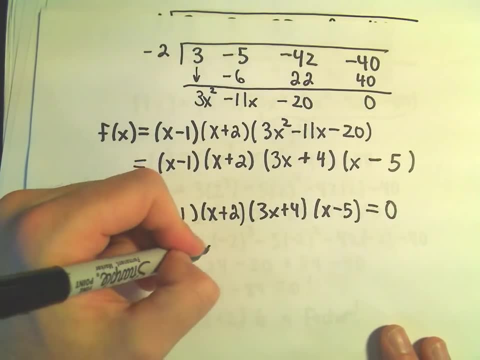 And then if we set each factor equal to zero, well, if we set x minus 1 equal to zero, we'll add and get x equals 1.. Since x plus 2 was a factor, we said that that means that negative 2 is a zero.